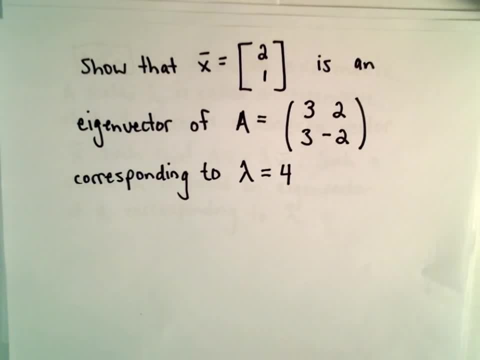 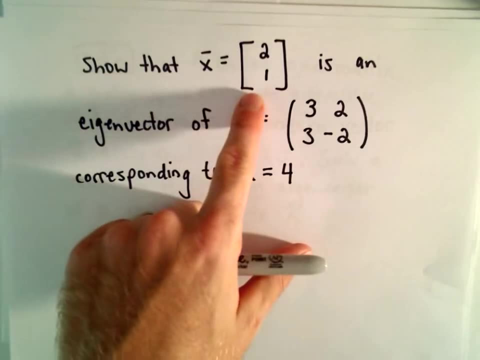 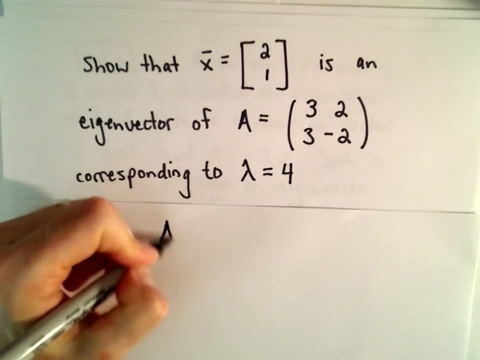 4. Okay, I'm not saying that this matrix A actually has other eigenvalues. We'll talk about that as well. This matrix also has other eigenvectors, and we'll talk about that in just a second. Okay, so really, all we have to do is we want to show, is the equation A. 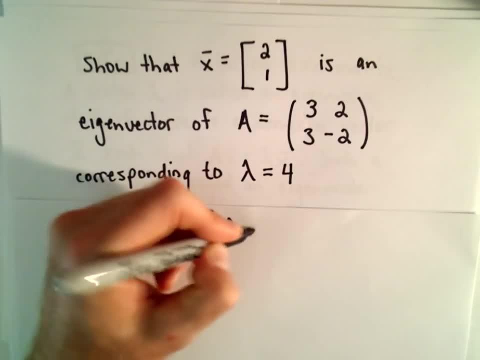 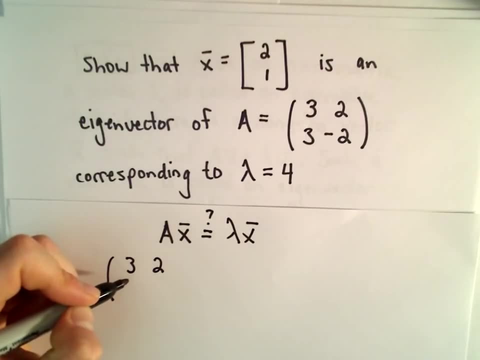 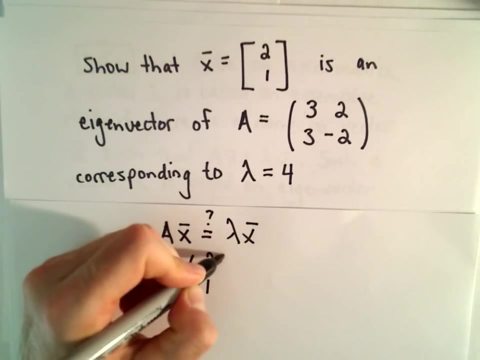 times x. does that equal? Does that equal, lambda times x? So not a lot to do here other than just a bit of arithmetic. So our matrix A has entries 3, 2, 3, and negative 2.. Again, our vector x has entries 2 and 1.. 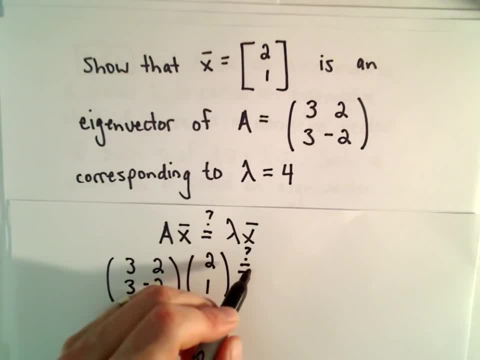 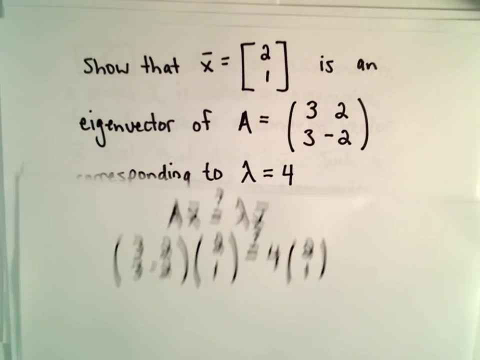 And I'm asking myself: well, is that going to be equal to the right side when we take lambda, which is 4, and again, multiply that by x? Well, it's going to be equal to the right side when we take lambda, which is 4,, and 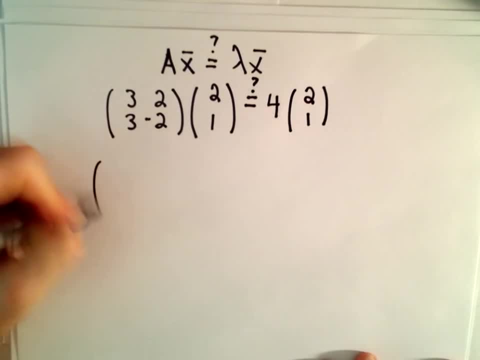 again multiply that by x. Well, it's going to be equal to the right side when we take lambda, which is 4, and again multiply that by x. Well, all we have to do is just a bit of arithmetic. So on the left side, we'll do our matrix multiplication: 3 multiplied. 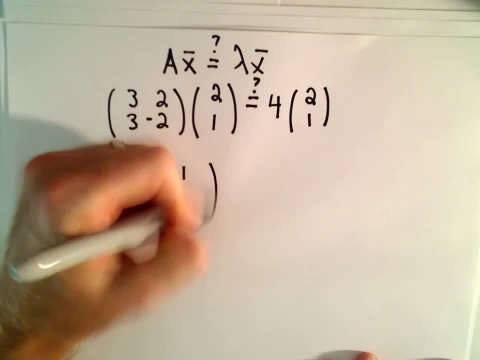 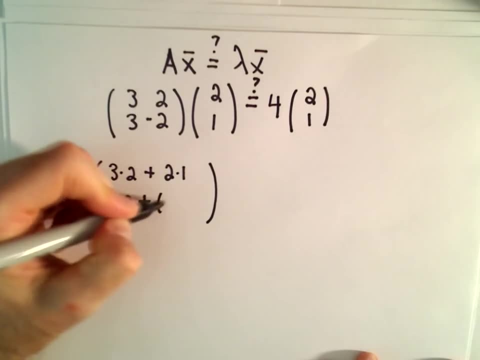 by 2 plus 2 multiplied by 1.. That'll be our first row, And then our second row. we'll have 3 multiplied by 2, plus then we'll take negative 2 multiplied by 1.. Well, on the right. 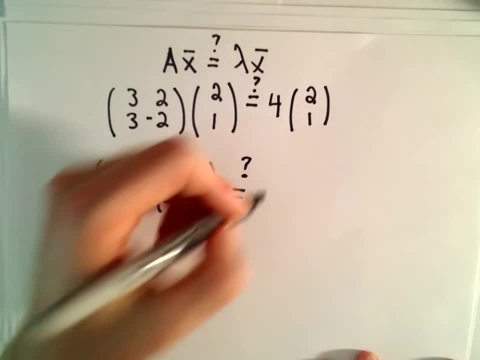 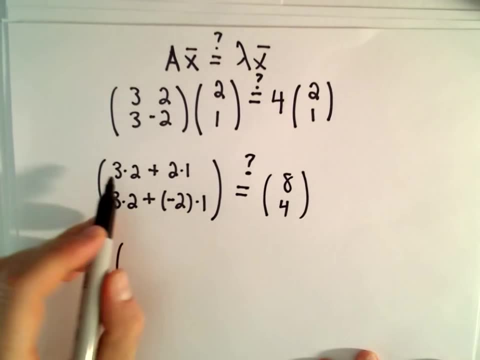 side, we just multiply our entries 2 and 1 by 4.. Well, 4 times 2 is 8, 4 times 1 is 4.. Well, on the left side, 3 times 2 is 6 plus 2 times 1 will give us 8.. 3 times 2 is 6, we'll. 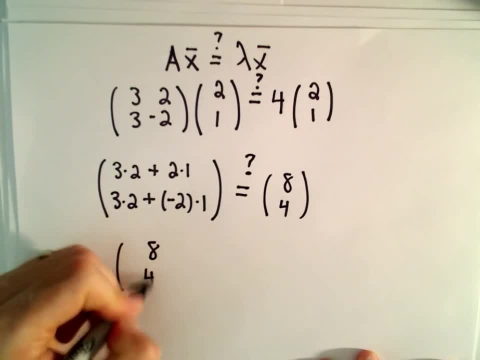 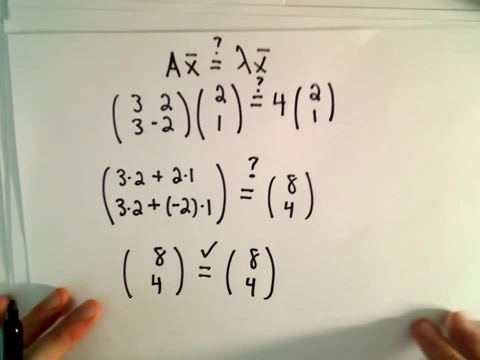 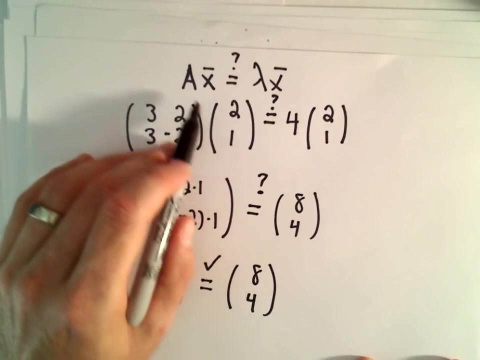 have plus negative 2.. So 6 minus 2 will give us 4.. Hey, that certainly does give us equality. So yes, in fact we would say that the vector with entries 2 and 1 is an eigenvector of. 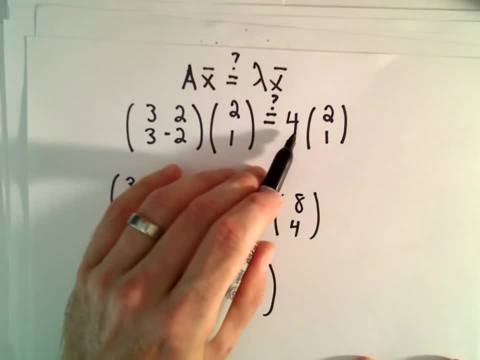 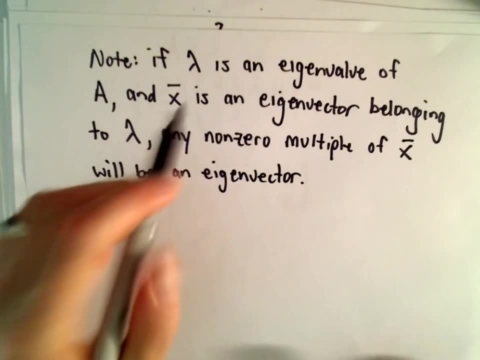 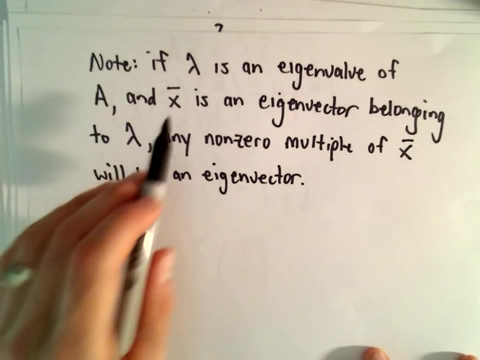 the matrix A corresponding to the eigenvector. Okay, so one other little remark here. If lambda is an eigenvalue of A- so we had, 4 was an eigenvalue of our matrix A, and x is an eigenvector belonging to lambda. so again,